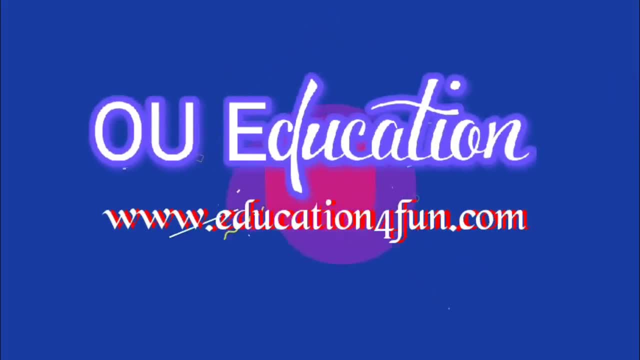 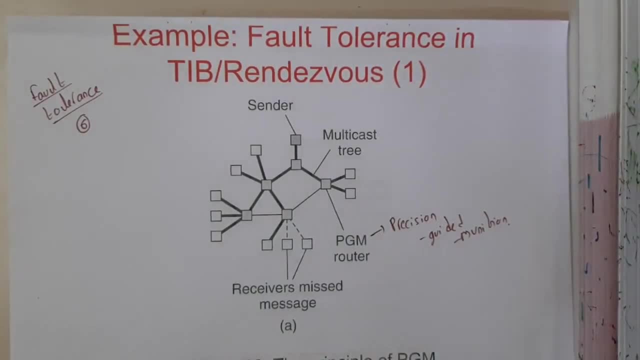 Hello guys, you're back with our next lecture. In this lecture, let us go through the concept of fault tolerance in coordination-based system. So I hope everyone knows about fault tolerance, right? So whenever a question is asked like this in particular system. so first of all, 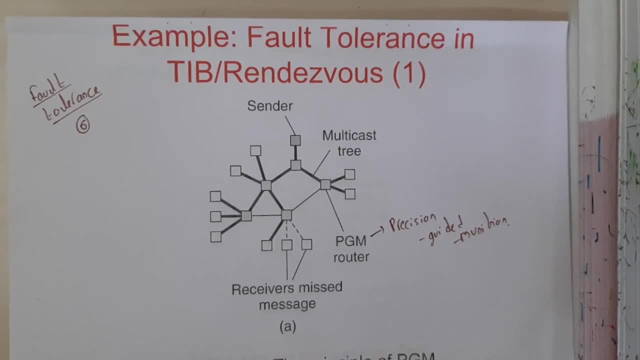 define fault tolerance and write about some points about fault tolerance and then you start explaining about: in this situation, guys, Because in that situation only your answer will be a bit lengthy, right? So we will be getting these kind of answers for LAPs only. So please make sure that. 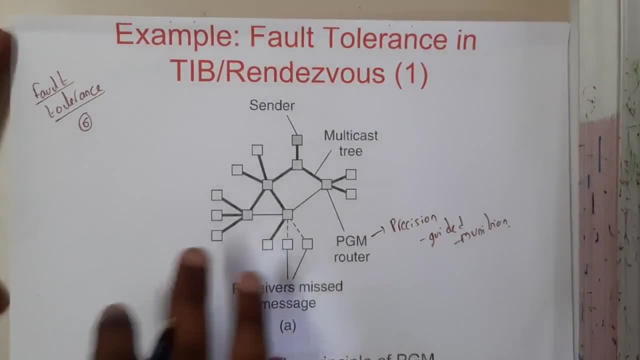 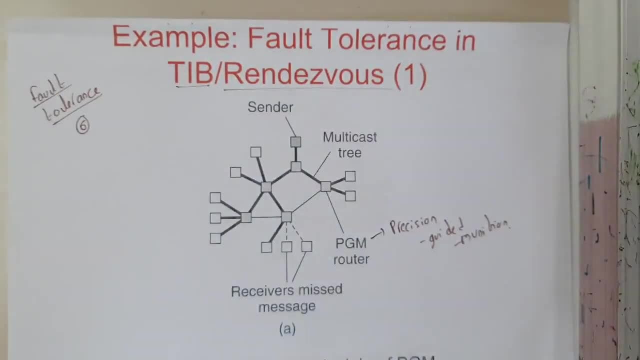 you are writing some introduction also for them, because it will be better for you, right? Yes, Okay, So here we are directly taking an example, guys. So we discussed about TIB. that is nothing but Renzowoo's system, right? Yes, So where the data is sending to a particular subscriber. 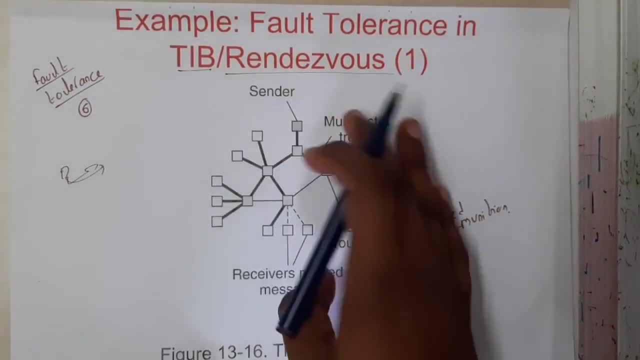 right, Yes, If you recall. yes, So if you draw that in the form of a tree, that tree is nothing but this. It will be looking like this guys, So that kind of thing. So if you draw that in the 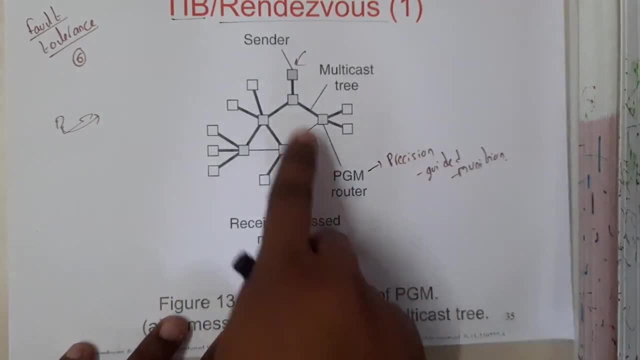 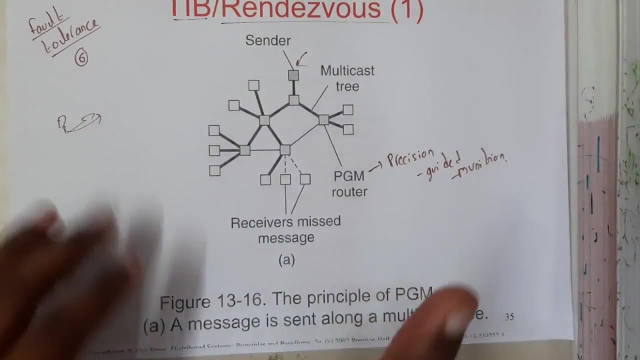 Okay, Yes, So here is our original sender, and here it is traveling to everyone the message. Okay, So slowly it is spreading, Okay, So assume that among the whole tree, one guy is not willing to take. So what will be the situation? He will be sending the negative acknowledgement, right, Or? 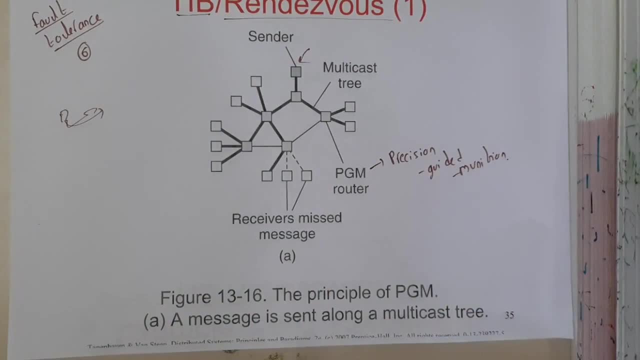 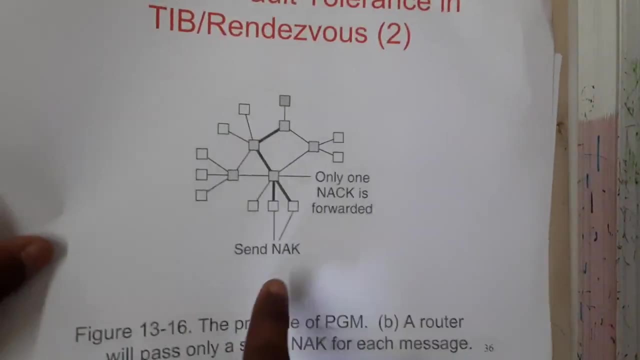 it is corrupted, He will be sending the negative acknowledgement that: okay, no, I don't want, or please resend me the file. Please resend me the file. Like that, there could be multiple situations, right? Yes, So in that situation he will be sending the message to someone above, So assume. 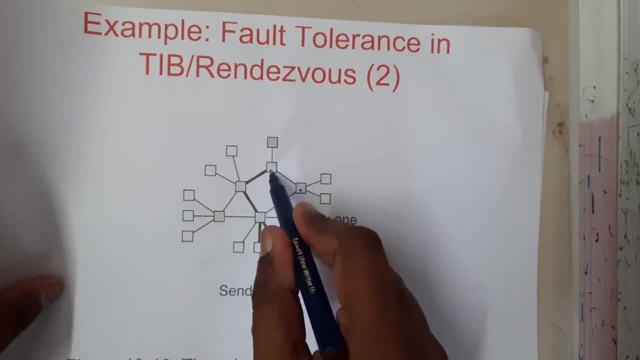 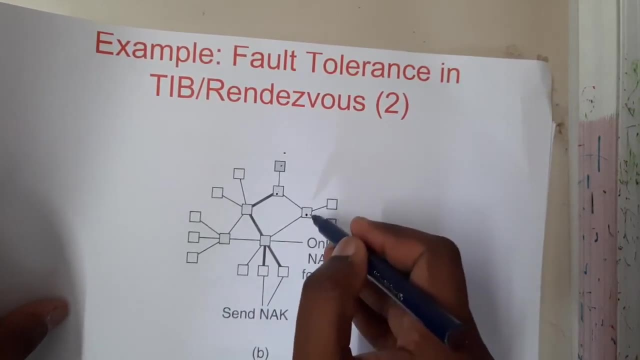 that this guy is not interested in the message, So he will be sending the message to him. This guy will be saying that my next guy is not interested to the sender. So the sender will be saying, okay, he don't want, Okay, It's okay, Or assume. 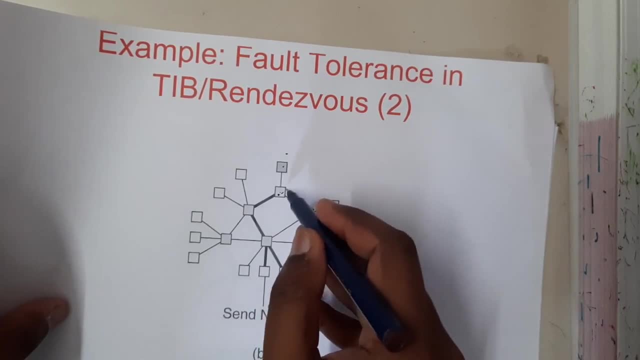 that there is a corrupted file. He will be saying to him: my file is corrupted, Please ask them to resend. So he will be asking him. So from here he will be getting resending the file. So in that. 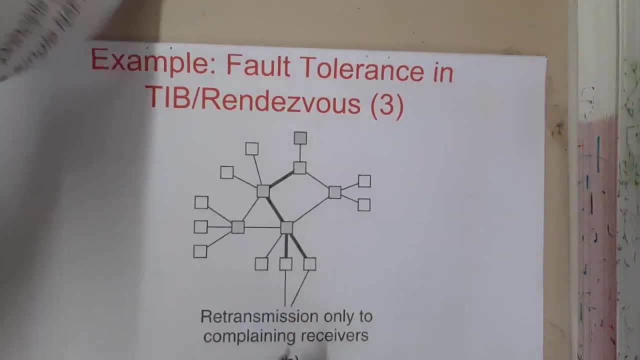 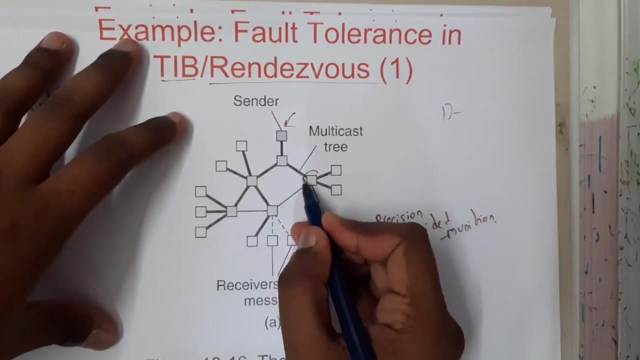 way, the resending and everything will be working, guys. So, basically, tolerance is nothing. but what is tolerance, guys? So whenever something goes wrong, the rest of the circuit should work perfectly. So if this node gone wrong, only this part will be lost and rest of the part will be.